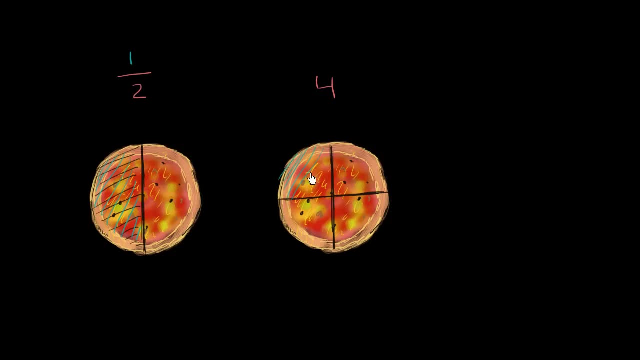 Well, I would eat this piece. You could imagine me eating this piece and this piece right over here. I've eaten the same amount of the pizza. Each of these pieces you could imagine got cut into two pieces when I cut the whole pizza. 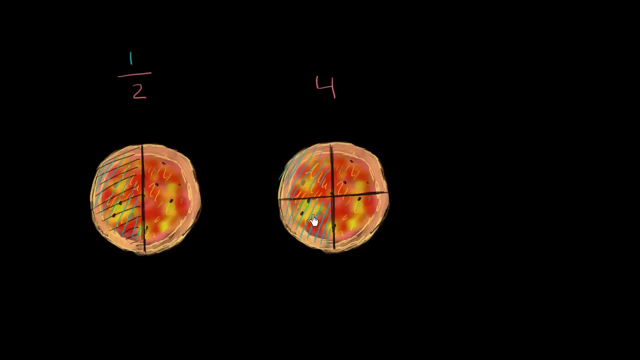 I could imagine the whole pizza this way, And so now I have to eat two slices of the four as opposed to one slice of the two, So I just ate two out of the four slices. So, even though I'm using different numbers here, 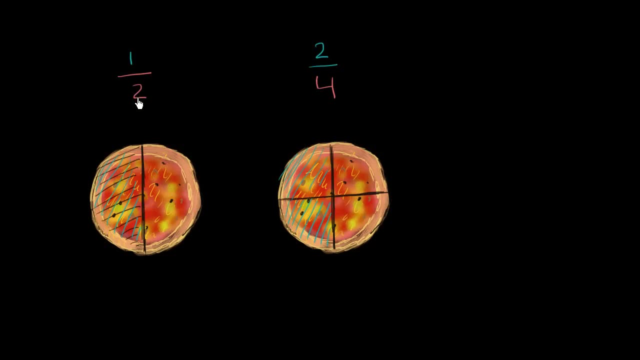 Here I'm using a 1 half or 1 in the numerator, a 2 in the denominator. Here I'm using a 2 in the numerator and a 4 in the denominator. These two fractions represent the same quantity. I ate the same amount of pizza. 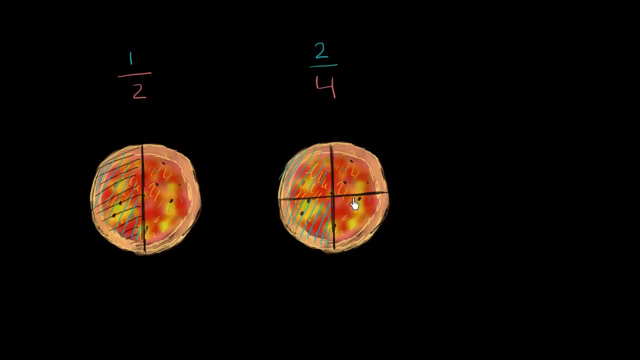 If I ate 2 fourths of a pizza, if I eat 2 out of 4. equal pieces, that's the same fraction of the pizza as if I eat 1 out of 2 equal pieces. So we would say that these two things are equivalent fractions. 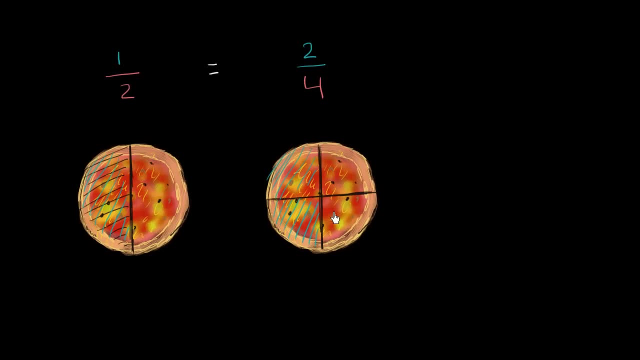 Now let's do another one like this: Instead of just dividing it into 4 equal pieces, let's divide it into 8 equal pieces. So now we could cut once like this: So now we have 2 equal pieces. Cut once like this: 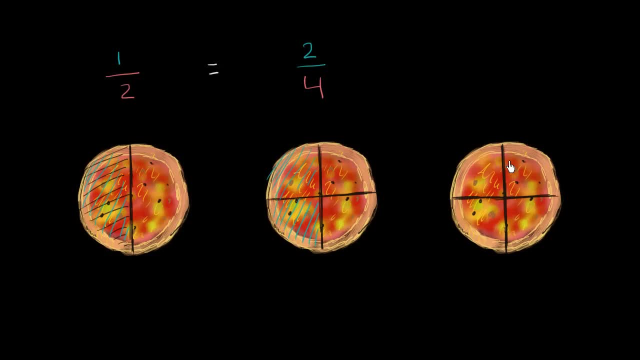 Now we have 4 equal pieces And then divide each of those 4 pieces into 2 pieces, So we'll cut those in. So here we have. so let's see, I want to make them equal pieces. Those don't look as equal as I would like. 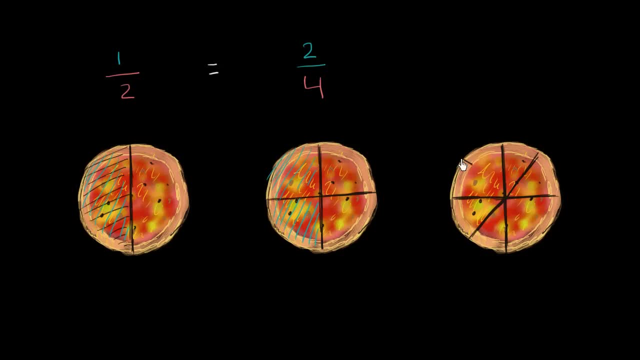 So that looks more equal And then that looks reasonably equal. So now, how many equal pieces do I have? I have 8 equal pieces, But let's say I wanted to eat the same fraction of the pizza, So I could eat all of these pieces right over here. 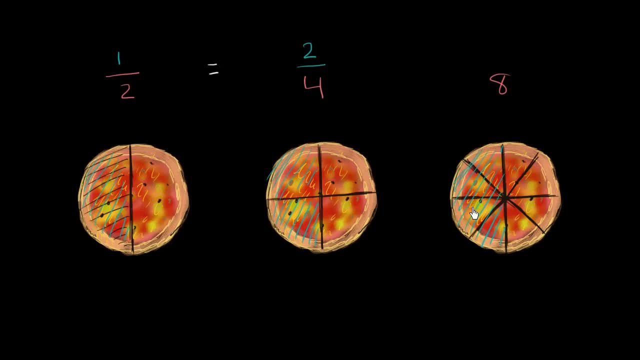 Well, how many of those 8 equal pieces have I eaten? Well, I've eaten 1,, 2,, 3,, 4 of those 8 equal pieces, And so, once again, this fraction 4 of 8, or 4 eighths.